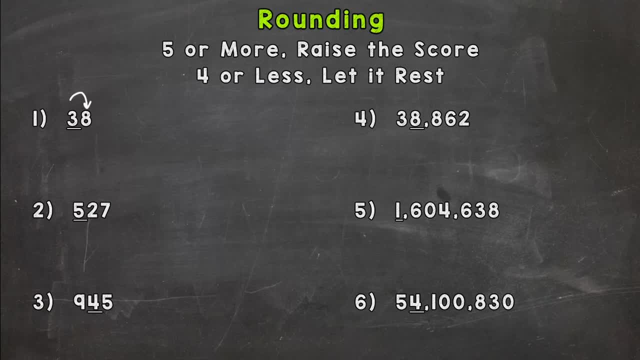 take a look next door. We have an eight. So does that tell the three to rest? Stay at three, stay at 30 or round up to 40.. Five or more raise the score. Well, eight is more than five, so we round up. So our rounded number would be 40 for. 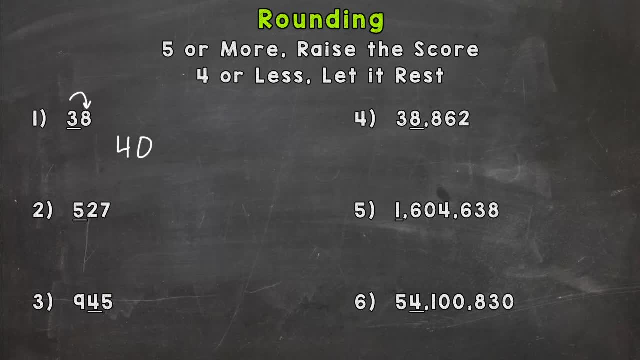 number one. Let's take a look at number two here: 527.. So we are rounding to the hundreds place. We are seeing if this number is closer to 500 or 600.. So let's take a look next door. This two is four or less. So we let the five rest. So the 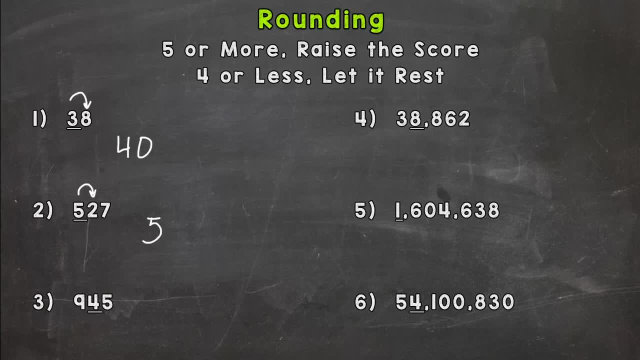 five stays the same and our rounded number is 500.. Right, This five stays the same and then everything to the right changes to a zero. So let's take a look at number three. here We're rounding the tens, place That four. So we look next door and we have five or more there. So we need to raise. 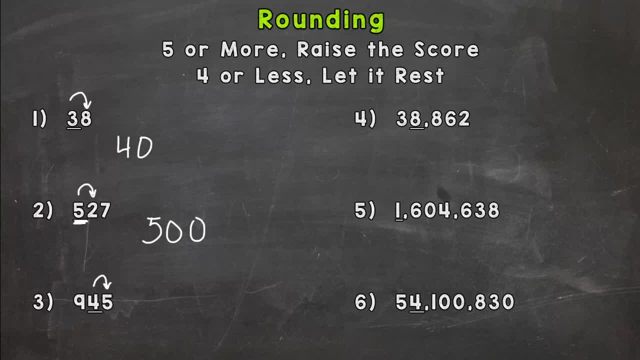 the score We need to round up to 950.. That four is going to change to a five Round up and then everything to the right of the underlined digit is changed to a zero. So let's take a look at number four. here We have 38,860. 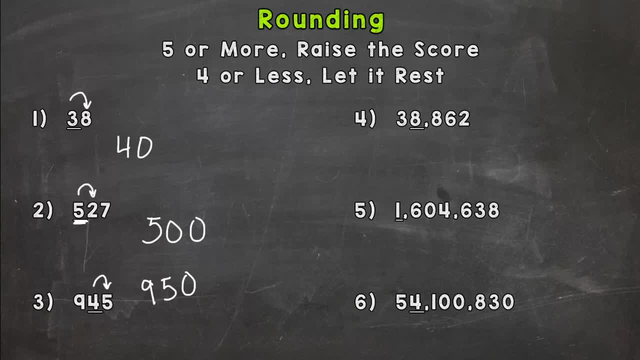 and then everything to the left of the underlined digit is changed to a six. So we're rounding up to 8,862.. What place is that eight in The underlined eight? Hopefully you're thinking the thousands place. So what we're doing here is we are. 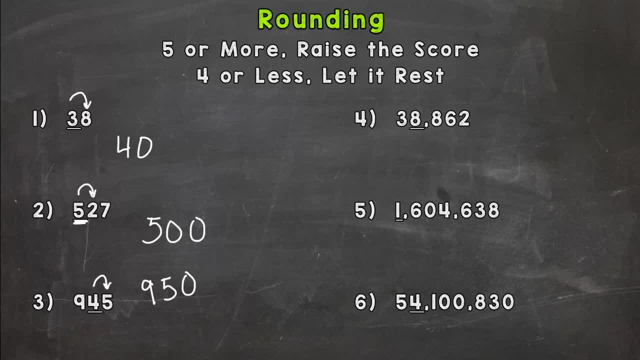 seeing if this number is closer to 38,000 or is it going to round up to 39,000.. So let's take a look next door. That eight is five or more, So it tells us that it's going to round up to 39,000.. So we keep everything to the left. the 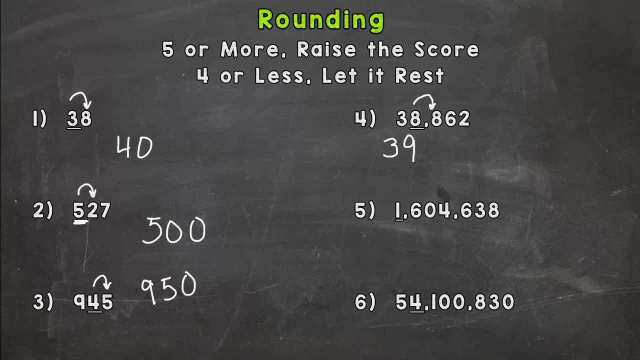 same. This eight is going to round up to a nine. and then what do we change everything to? To the right of the underlined digit- Hopefully you're thinking zeros- So that number is closer to 39,000 than it is 38,000. It. 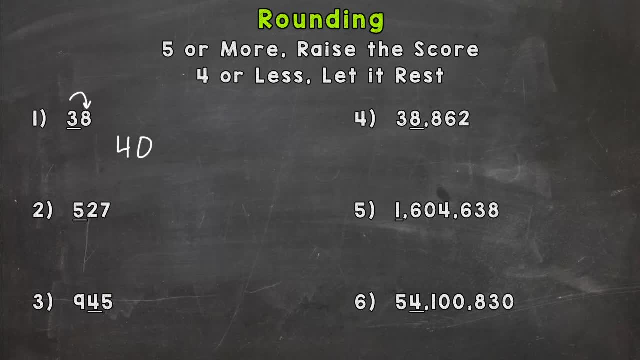 number one. Let's take a look at number two here: 527.. So we are rounding to the hundreds place. We are seeing if this number is closer to 500 or 600.. So let's take a look next door. This two is four or less. So we let the five rest. So the 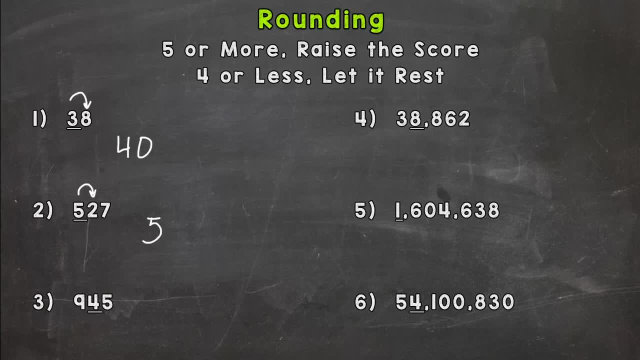 five stays the same and our rounded number is 500.. Right, This five stays the same and then everything to the right changes to a zero. So let's take a look at number three. here We're rounding the tens, place That four. So we look next door and we have five or more there. So we need to raise. 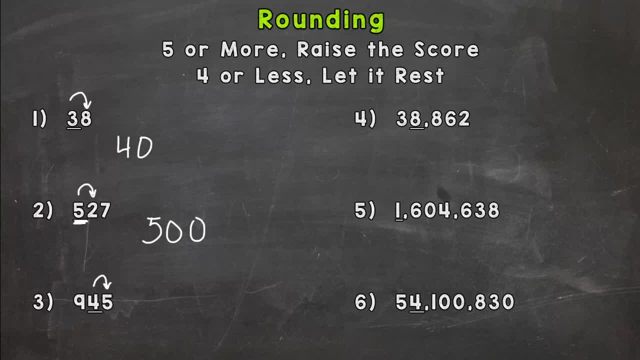 the score We need to round up to 950.. That four is going to change to a five Round up and then everything to the right of the underlined digit is changed to a zero. So let's take a look at number four. here We have 38,860. 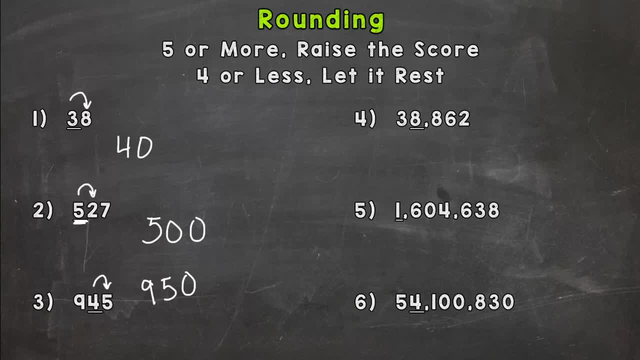 and then everything to the left of the underlined digit is changed to a six. So we're rounding up to 8,862.. What place is that eight in The underlined eight? Hopefully you're thinking the thousands place. So what we're doing here is we are. 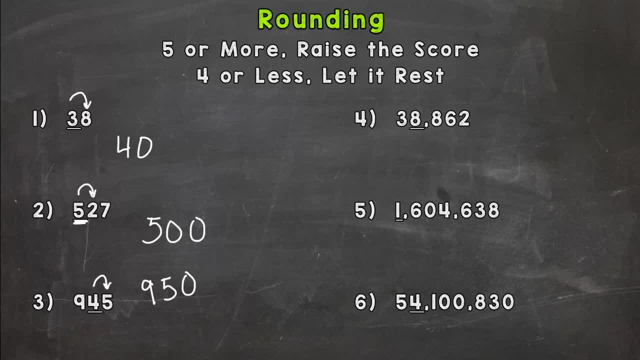 seeing if this number is closer to 38,000 or is it going to round up to 39,000.. So let's take a look next door. That eight is five or more, So it tells us that it's going to round up to 39,000.. So we keep everything to the left. the 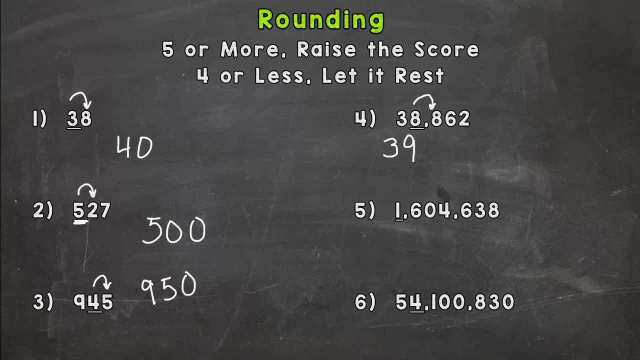 same. This eight is going to round up to a nine. and then what do we change everything to? To the right of the underlined digit- Hopefully you're thinking zeros- So that number is closer to 39,000 than it is 38,000. It. 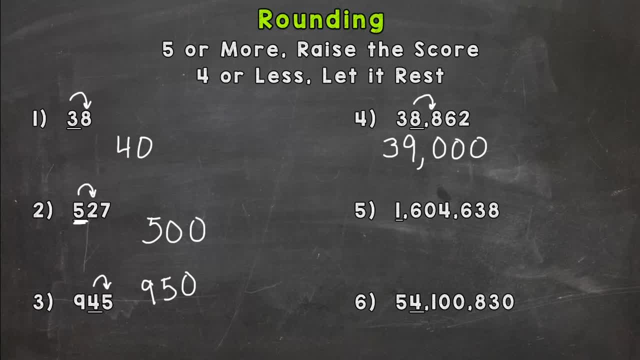 rounds to 39,000.. Let's take a look at number five. here We have a one underlined and that one is in the millions place. So we are going to take a look next door to see if this number rounds up to two million or will round.